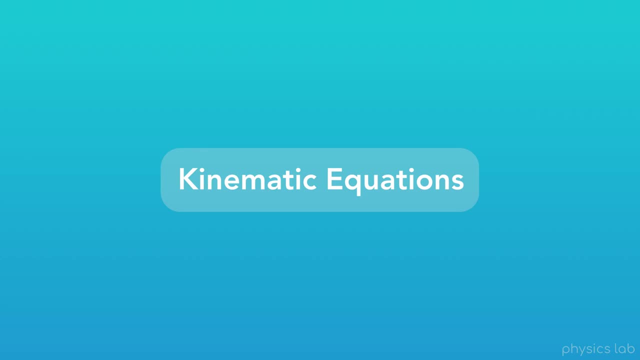 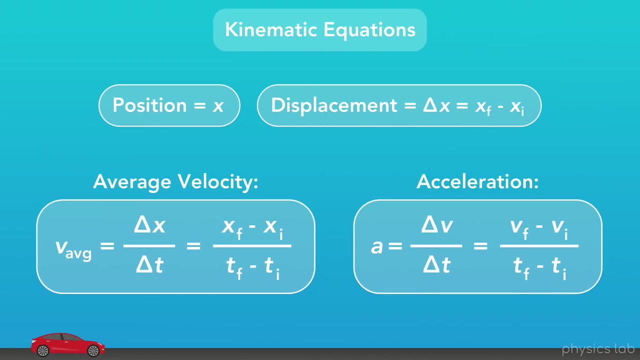 the linear motion of objects and see how we can apply them to both horizontal and vertical motion. Just as a quick reminder, here are the kinematic equations for position, displacement, velocity and acceleration that we learned in the last video. These equations are what we might call. 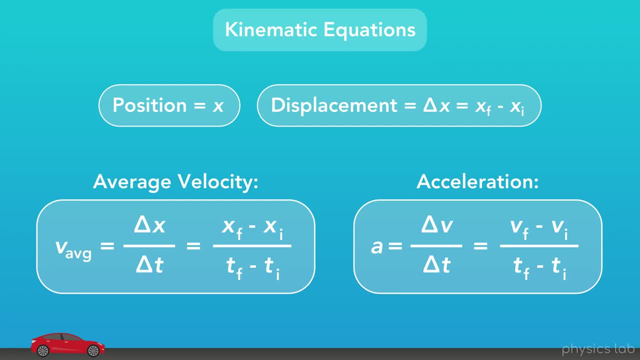 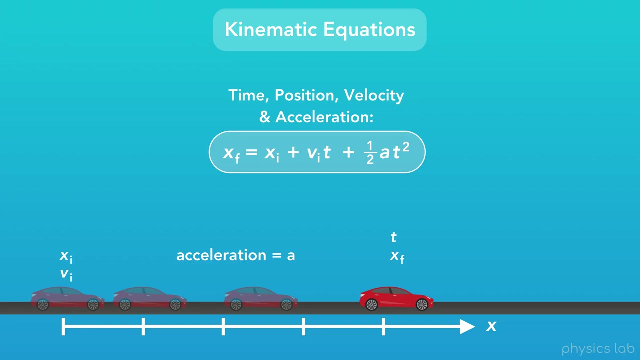 the definitions of position, velocity and acceleration. The next two kinematic equations that we'll learn are really useful and they combine all three of these. So this first equation includes the variables for time, position, velocity and acceleration, And for an object that's accelerating, this equation helps us find the object's position. 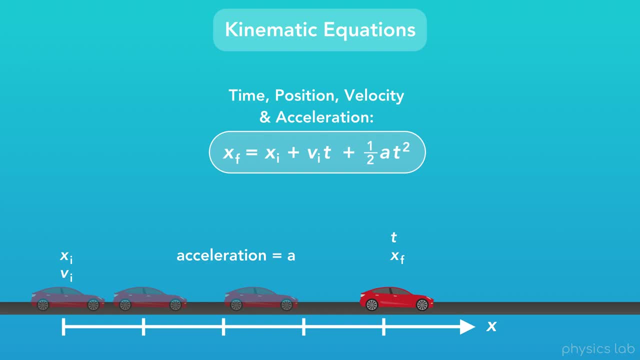 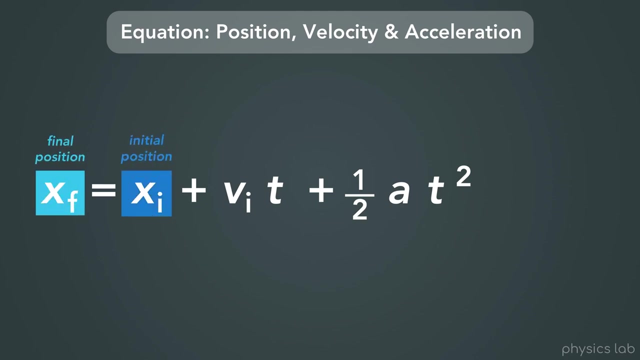 at any point in time by using the initial position, the initial velocity, the acceleration and how long it's been accelerating. for Let's take a closer look. So in this equation, xf stands for final position, xi is the initial position, vi is the initial. 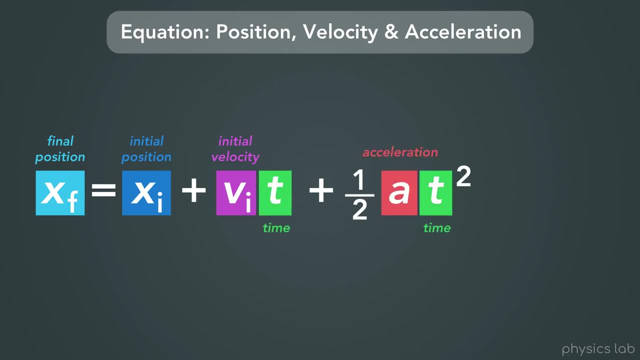 velocity. t is the time and a is acceleration. Something to note here, which we covered in one of the basics videos, is that when we have two variables next to each other with nothing in between them, it means we have to multiply them together. So here we have initial velocity times. 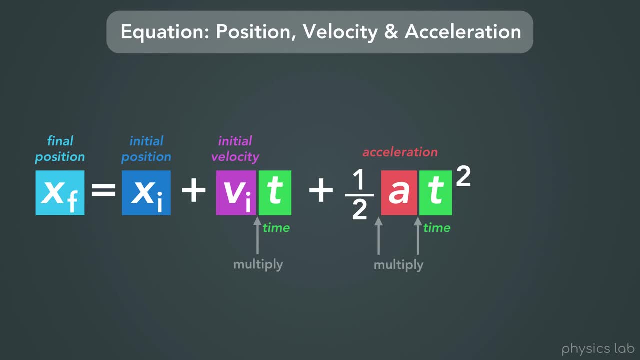 time and we have one half times acceleration times time squared. Another important thing to point out is that this equation only has the variable t for time. It doesn't have a delta t for change in time and there's no initial time and final. 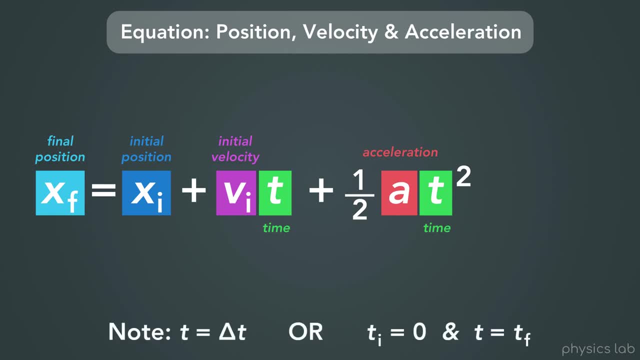 time. The thing to remember is this: For equations that only have a t by itself, the t really means delta t or change in time. Or we could also think of it this way: We assume the initial time is just 0, and t is equal to the final time, which is the time point that we care about, the time point we're 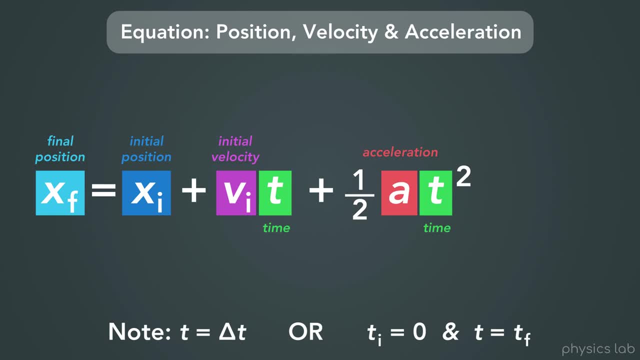 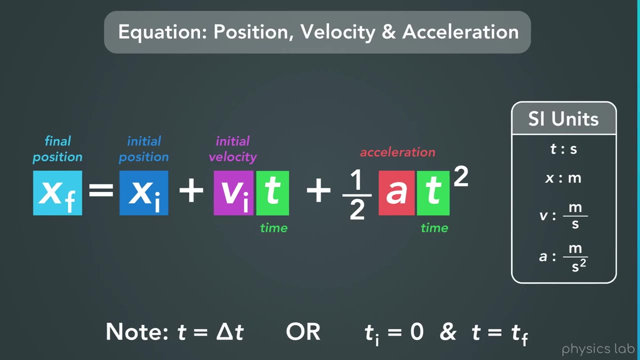 plugging in to find the object's position. And here are the SI units that we use for this equation: Time is in seconds, position is in meters, velocity is meters per second and acceleration is meters per second. squared, Alright. now the last kinematic equation that we'll learn for linear motion is this one: 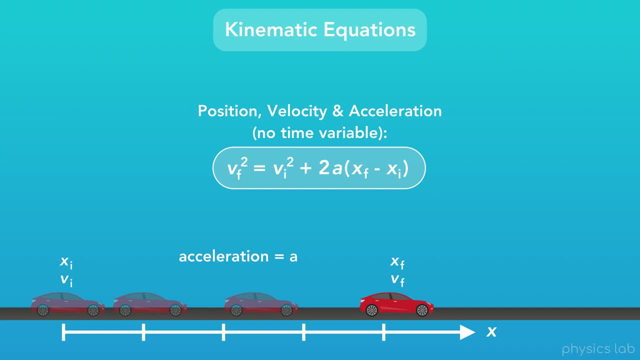 This equation relates the position, velocity and acceleration of an object, but it doesn't include the variable for time, which is pretty interesting because time is a fundamental part of kinematics. This equation is actually made by combining and rearranging a few other equations in order to get 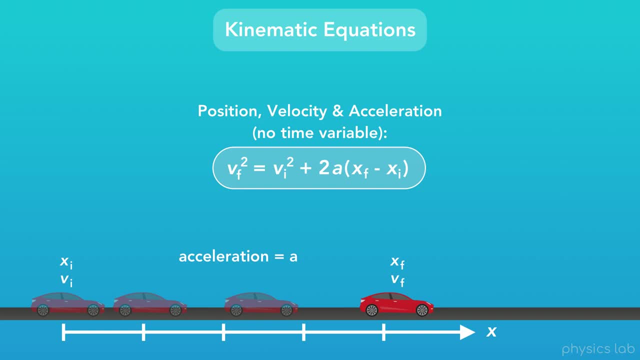 rid of the variable for time, which makes it really useful for certain problems where we don't know anything about time. So, for an object that is accelerating, like this car, this equation will help us find the final velocity of the object, based on its initial velocity, its acceleration and its change in. 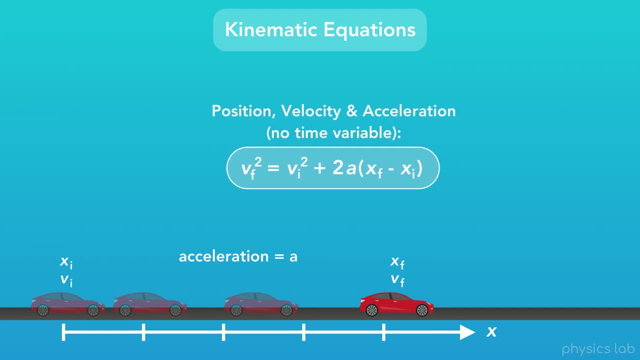 position. This looks very similar to the equation we learned for acceleration if we had rearranged the variables like we mentioned in the last video. So with the equation on the left, we're using the change in time, which is the part in parentheses, and with this new equation on the right, we're 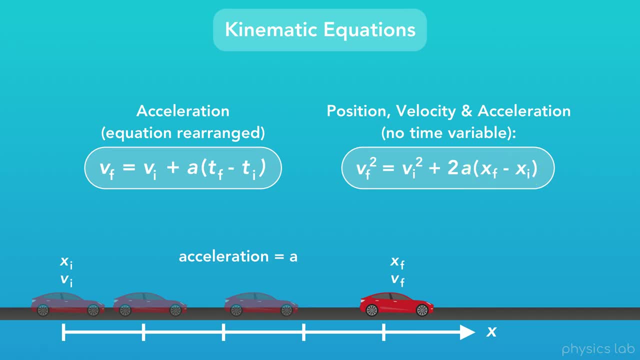 using the change in position. To put that into words, the left equation can tell us the car's velocity based on how much time the car has been accelerating for, and the right equation can tell us the car's velocity based on how much distance the car has been accelerating over. So let's take 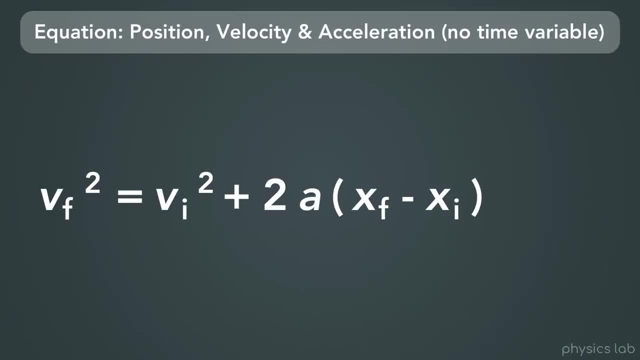 a closer look at the variables in this new equation. v, f stands for final velocity, vi is initial velocity, a is acceleration, xf is final position and xi is initial position. And don't forget, multiplication is implied in these two spots. 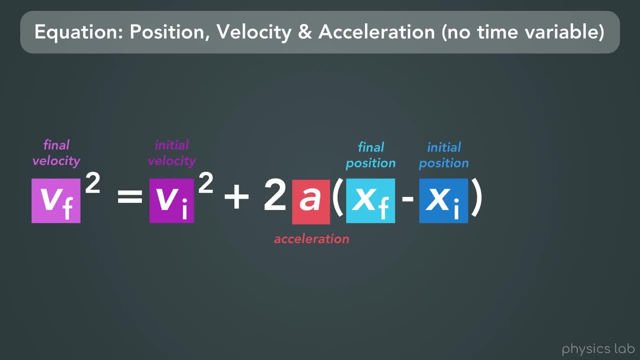 As a whole. this equation says that for an object the final velocity squared is equal to the initial velocity squared plus the initial velocity squared, two times the acceleration times, the change in position, or the final position minus the initial position. And here are the SI units for the variables in this equation: 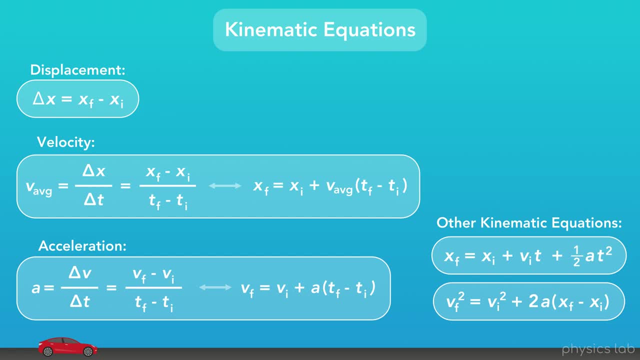 Awesome. so now we have a nice list of kinematic equations that we can use to solve problems, which we'll work through more in later videos, And don't worry if this seems like a lot here. you don't have to memorize it. All of these are on your equation sheet. 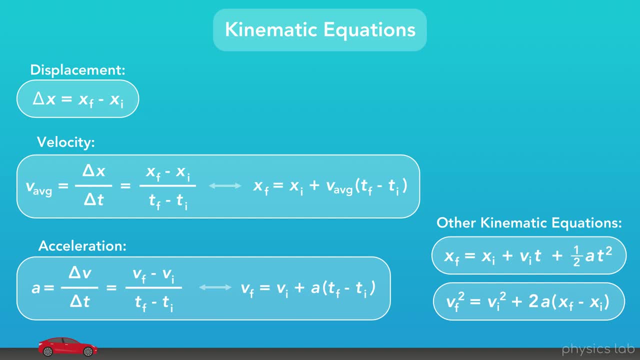 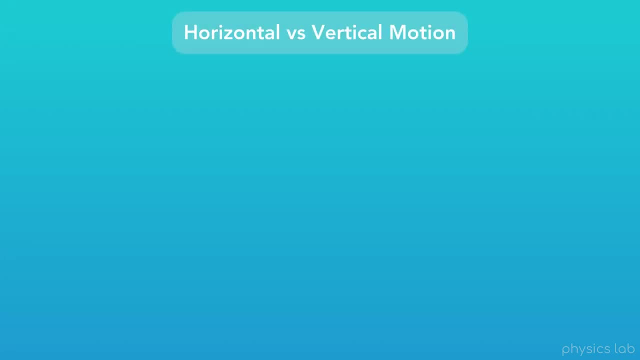 and the variables are defined there, so you'll know what they mean. Now, before we wrap up with kinematic equations, there's one more thing we need to cover, and that's the variables that we use for horizontal and vertical motion. So we're 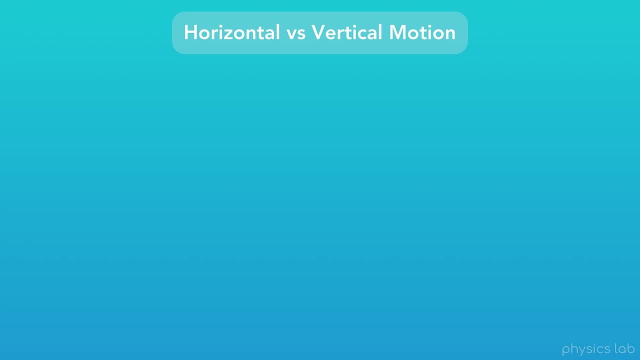 learning about linear motion or motion along a straight line, and mostly we've talked about a car driving along a road, which would be horizontal motion, But we can also have vertical motion, which would be horizontal motion, But we can also have vertical motion, which would be. 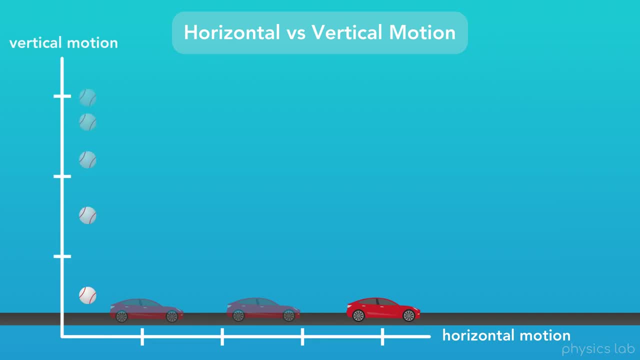 vertical motion, which would be horizontal motion, But we can also have vertical motion, which would be horizontal motion, But we can also have vertical motion, like if we dropped a ball from some height and let it fall down. The car and the ball are both examples of linear motion. 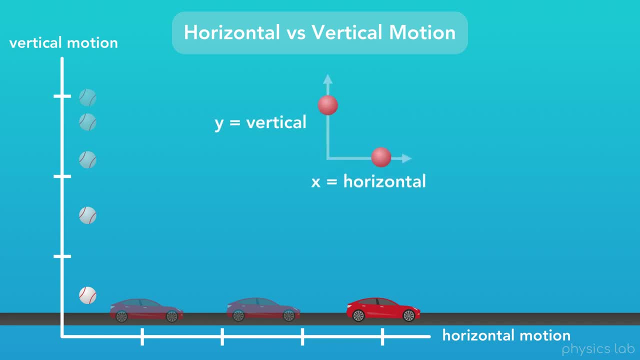 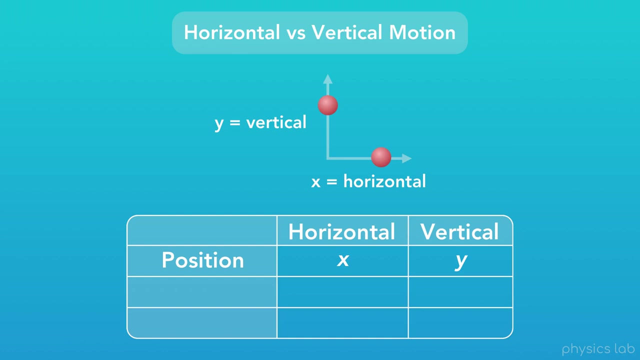 but they're in different directions. In physics, we typically use x to represent horizontal motion and we use y to represent vertical motion. So, just like we've been using x to represent horizontal position, we're going to use y to represent vertical position, or the height of an object. 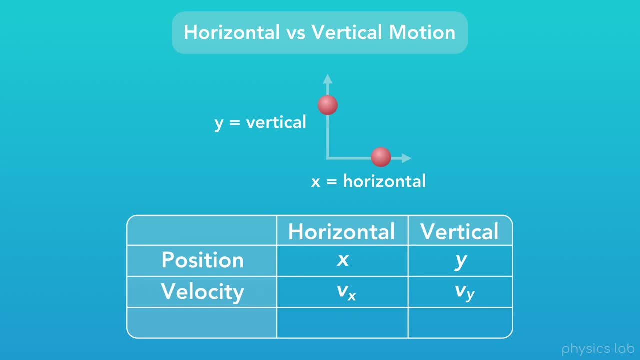 And sometimes we'll use x and y as subscripts to label the direction of something. We can use v with x as a subscript to mean velocity in the horizontal direction, or v with y as a subscript to mean velocity in the vertical direction. Likewise, ax would mean horizontal acceleration and ay would mean vertical acceleration. 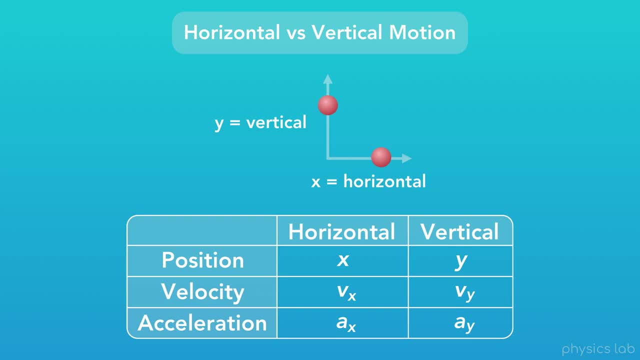 Now, when you look at this model, you'll notice that there are a lot of variables that we need to look at. to organize it this way, At least for me, it kind of feels like position should have its own variable, like p, and then we would use x and y as subscripts, just like velocity and acceleration do. 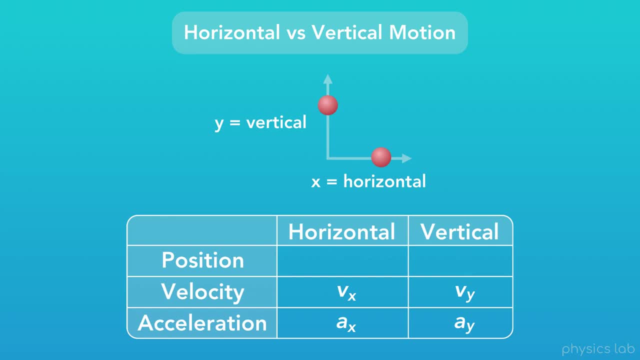 Well, the variable p is already taken, but you'll actually find in some places that people use the variable s to represent position, But in most cases I've seen everyone use x and y to represent position. so that's what we're going to do in this course. 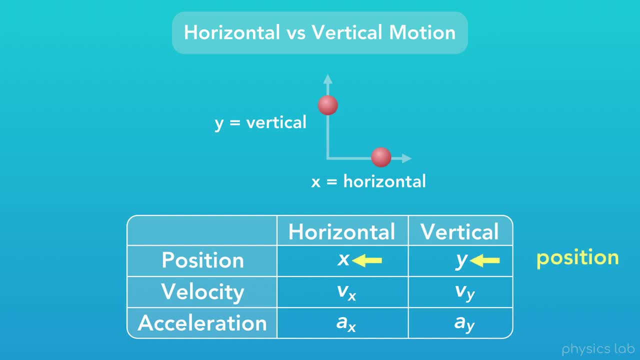 The takeaway here is that when they're the actual variables, x and y mean horizontal and vertical position, But when they're subscripts next to a variable, x and y are telling us the direction of that variable, like velocity or acceleration. So what does this mean for our list of kinematic? 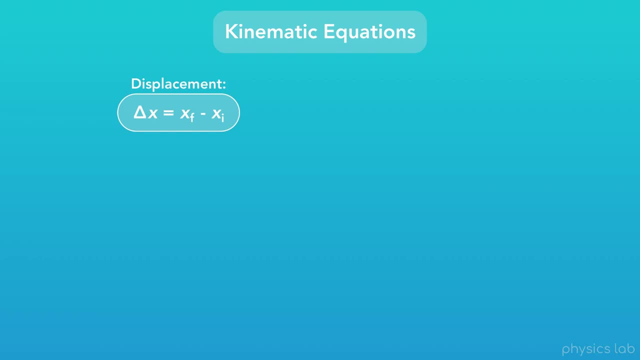 equations that we've put together. Well, it means we actually know twice as many equations as before without even learning them. Every equation can be applied to either horizontal or vertical motion just by using x or y. The equation we learned for displacement uses x for horizontal displacement. 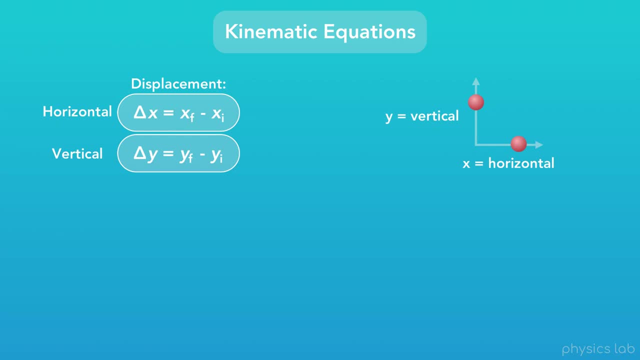 But if we use y instead of x, now we have an equation for vertical displacement. Here's our equation for average velocity that uses x, And again, if we use y instead of x, we have an equation for vertical average velocity. Notice how we've added x and y as subscripts for the average velocity variables to label them. 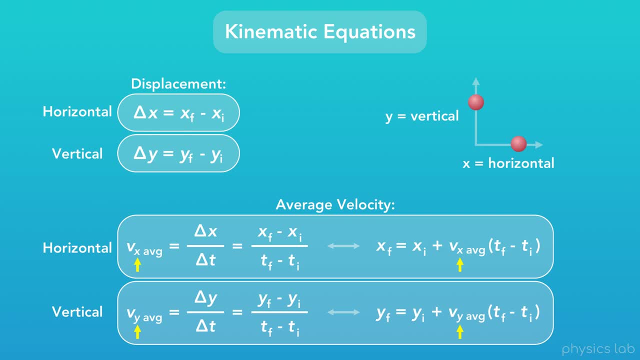 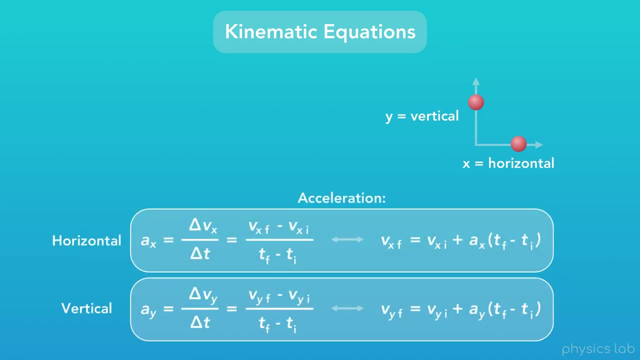 as average velocity in the horizontal or vertical direction, And we can do the same thing for our equation for acceleration. Here all the variables for velocity and acceleration get their own vertical speed subscript, x or y to label the direction. However the variable t for time does not. 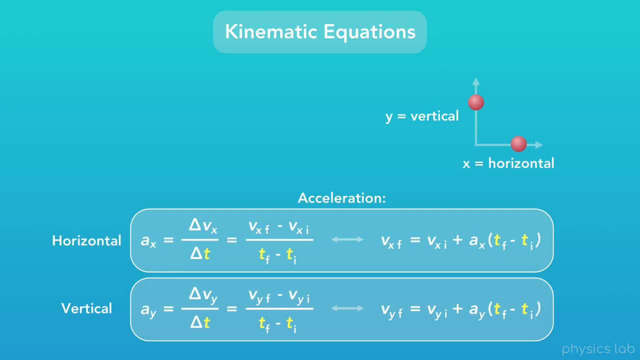 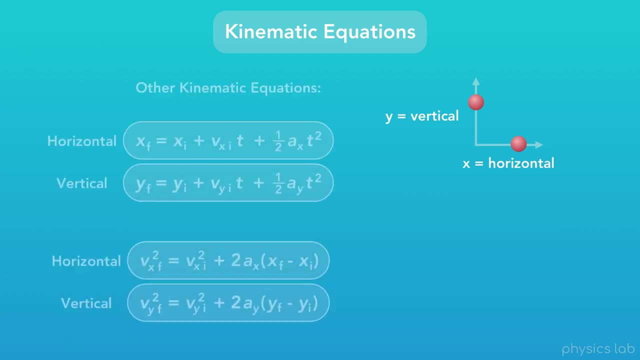 get an x or y subscript, because time applies to all motion. Time can't be horizontal or vertical. And finally, here are the last two kinematic equations that we learned, And again each one has a version for horizontal or vertical motion, just by using either x or y. So to wrap up this section, here's what I 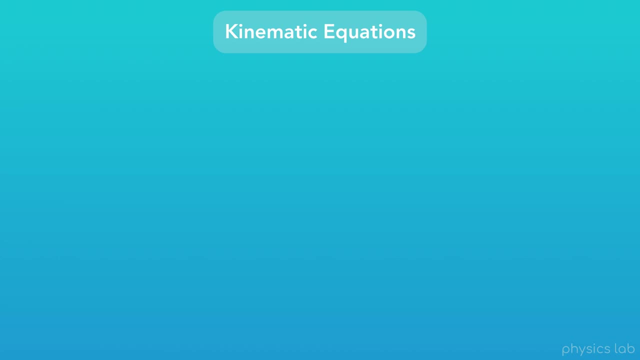 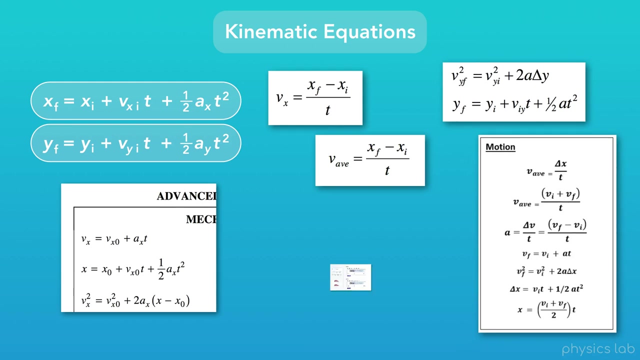 want all of you to take away from this. Different physics equations are going to show up in this course, in your class, in other online videos, maybe on a website where you do your homework, or wherever, And all of those equations might look. 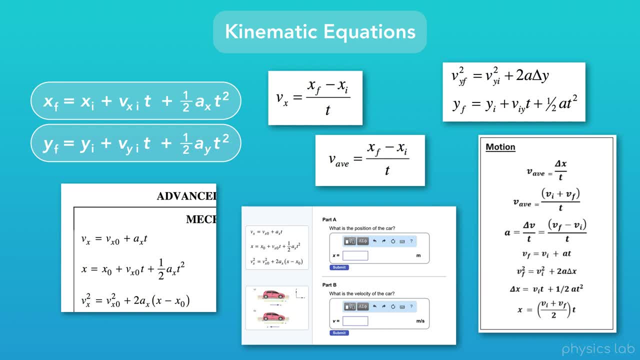 just slightly different from each other. They might have different subscripts or they might just be rearranged, And it can definitely be annoying, especially when you're learning these for the first time. But don't worry about all of that. All you need to know is what. 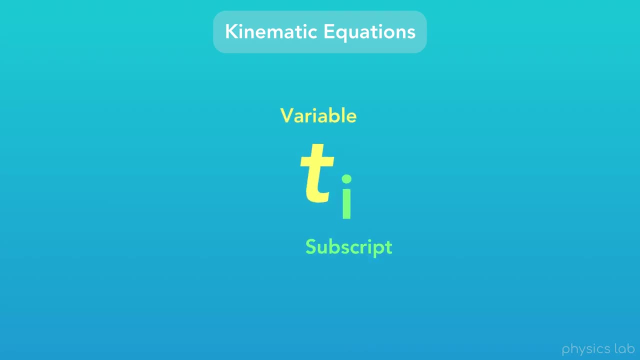 each variable means and what each subscript means. That way you'll understand how to use any equation, even one that you haven't seen before. So just to reiterate, the variables in an equation are the large letters and the subscripts are the smaller letters at the bottom right of the variable. We can 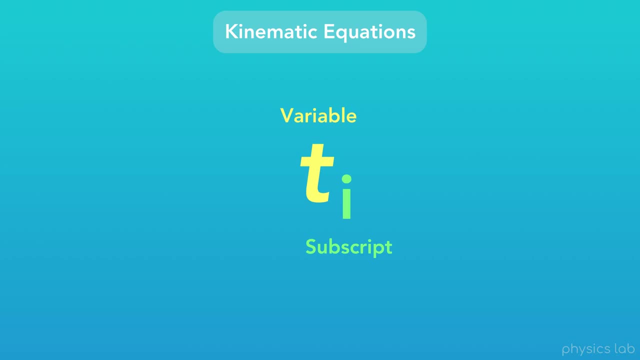 think of a subscript as a label, And a variable can also have more than one subscript. So for the kinematic equations, here are the variables that we'll use: t is time, As variables. x and y mean position, v means velocity And a means acceleration, And for the 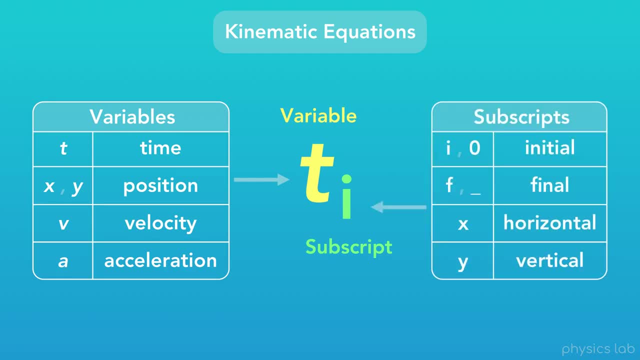 subscripts. i means initial, Or instead you might see a 0,, which means time 0. And it's also sometimes called not I and 0 both mean the same thing. f means final, And if there's no subscript it might also mean final. You would see variables. 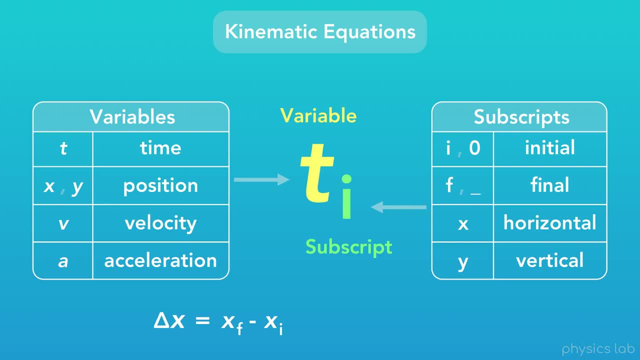 with the subscripts i and f in an equation, Or instead you would see variables with a subscript 0, and then one with no subscript. These are sort of paired together, Then x as a subscript x And the subscript y as a subscript y. These are sort of. 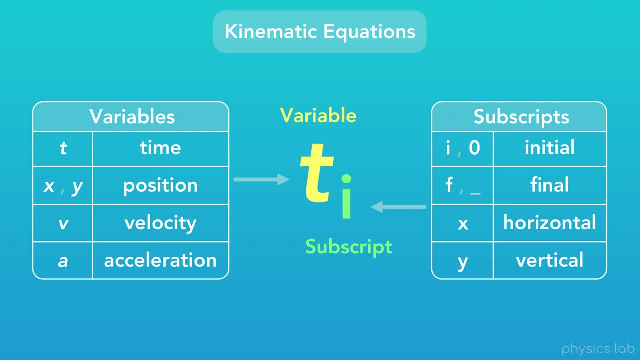 means the horizontal direction and y, as a subscript, means the vertical direction. And last, it's not a variable or a subscript, but remember that this little triangle is delta and it means the final value minus the initial value or the change in that value. And again, this might seem like a lot to remember, but 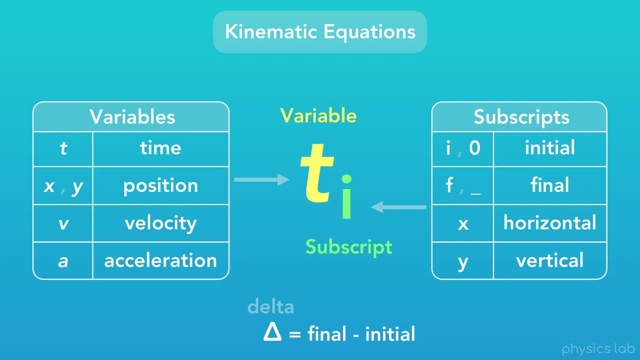 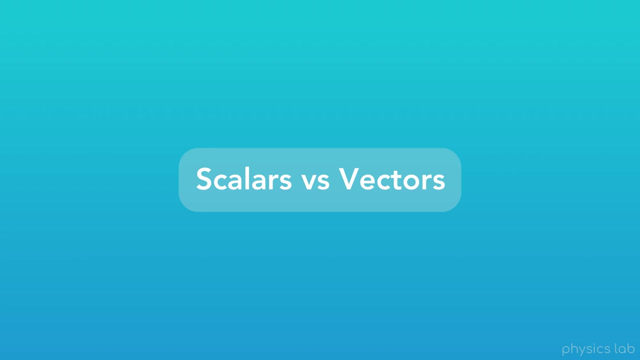 don't worry, the equation sheet for this course will have everything on it. This video is meant to introduce these equations, but we'll get a lot more comfortable with them as we start doing practice problems. So next up, let's talk about scalars and vectors. A scalar is a quantity that only tells you the 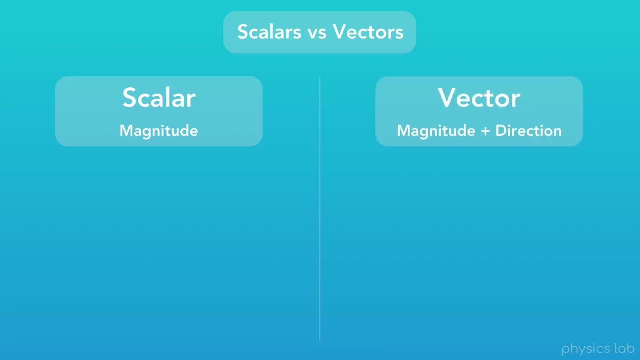 magnitude, and a vector is a quantity that tells you both the magnitude and the direction. So what does that mean? Well, scalars are what we're mostly used to. For example, 6 miles is a scalar quantity and 12 meters per second is a scalar quantity. 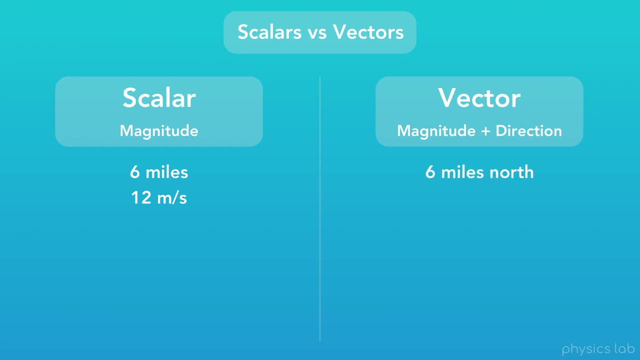 On the other hand, 6 miles north would be a vector, or 12 meters per second to the right would also be a vector. That's because they tell us the magnitude, like 6 miles, as well as a direction, like north. 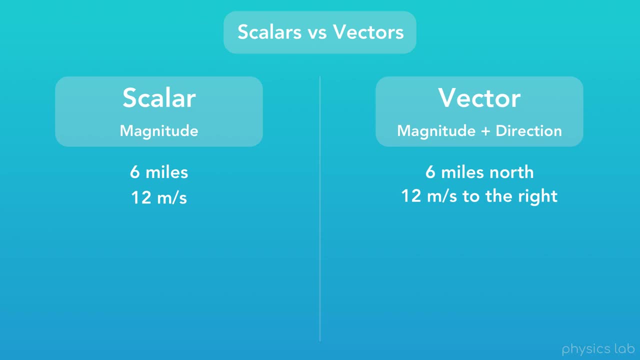 If you take a scalar quantity and add a direction to it, you turn it into a vector. Also, we've mentioned the words distance and displacement. The difference between them is that distance is a scalar and displacement is a vector, And it turns out this is the difference between speed and velocity. 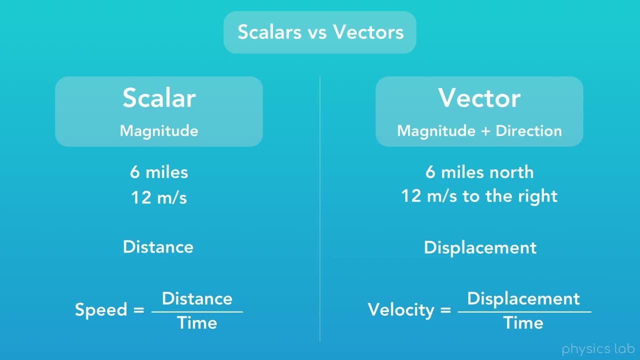 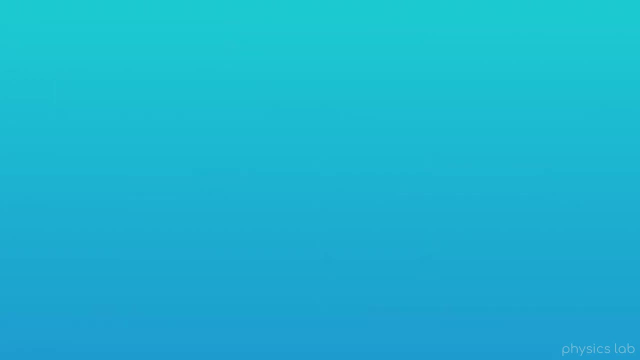 Speed equals distance over time, which makes it a scalar, while velocity equals displacement over time, So it's a vector. Let's take a look at the difference between distance and displacement. Here's our friend Mike. If Mike starts here and he travels 5 meters, where is he now? 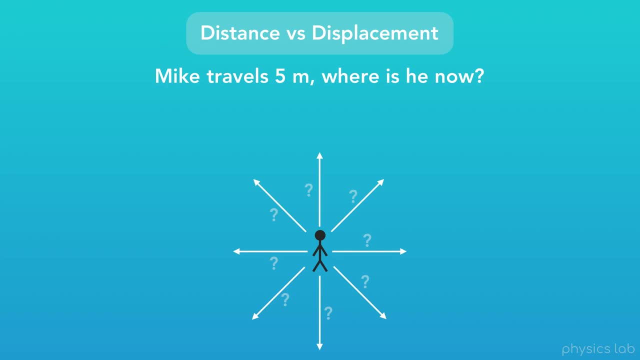 Well, it's not possible for us to know because we weren't given a direction. We were given a distance which is a scalar. Now, instead, say, we have a compass and we're told Mike travels 5 meters west. That's a vector. 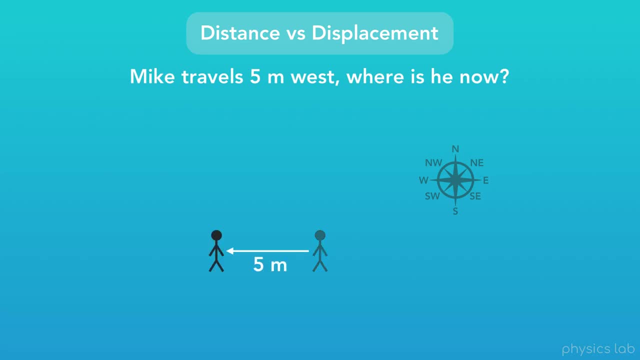 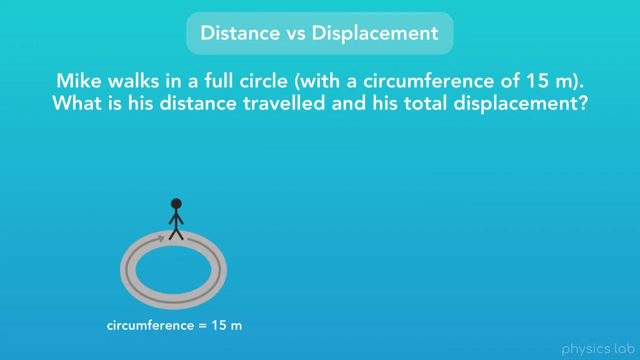 Now we know exactly where he is Here. we were given a displacement, which is a vector, and it includes both the magnitude and the direction. Think of it as taking a distance value and adding on a direction. Here's another important distinction between distance and displacement. 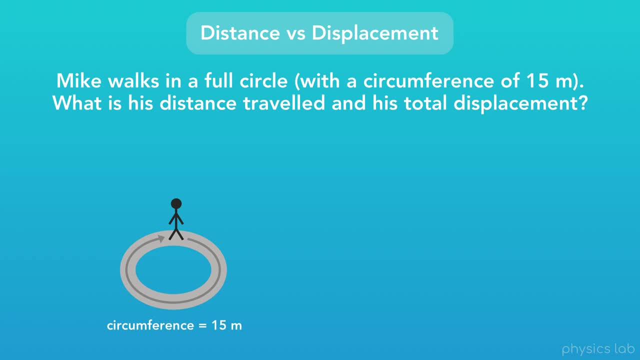 Here's Mike again. Let's say that Mike walks in a full circle with a circumference of 15 meters and ends up right where he started. What is his distance traveled and what is his total displacement? Well, his distance traveled, which is the actual path that he covered while he was walking. 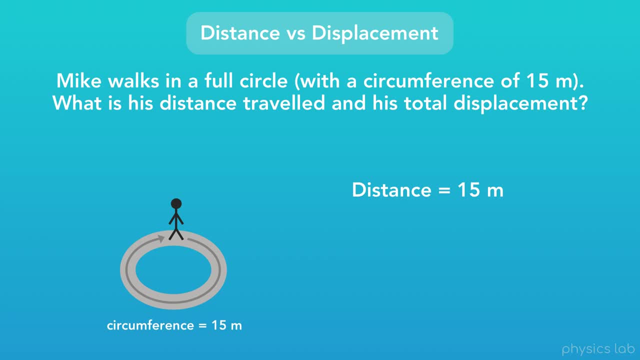 is 15 meters. That's the circumference of his circle, or the length of his path. However, his total displacement during this journey is zero. Why is that? Well, remember our equation for displacement: 0.. 0.. 0.. 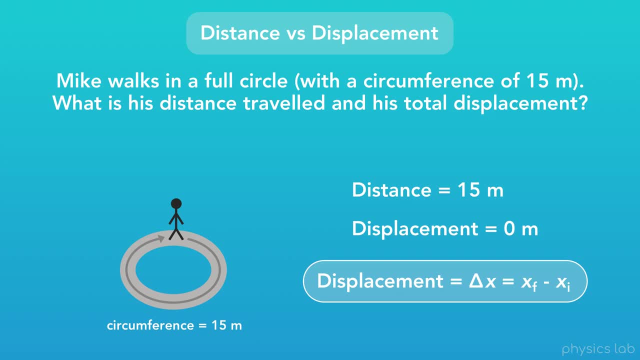 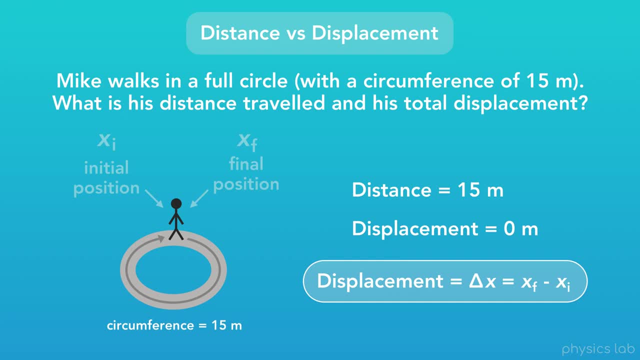 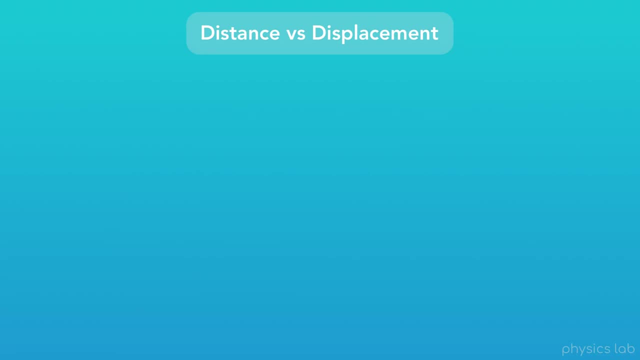 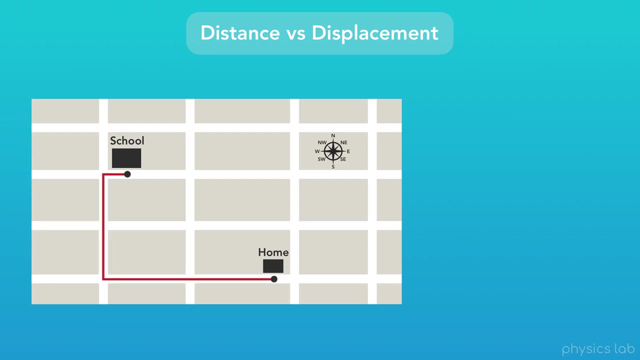 So his final position and his initial position are the same, and that gives us that the displacement is zero. Let's look at this another way. Let's say you're driving from your home to your school. There's different paths you could take, but let's say you drove to school like this: 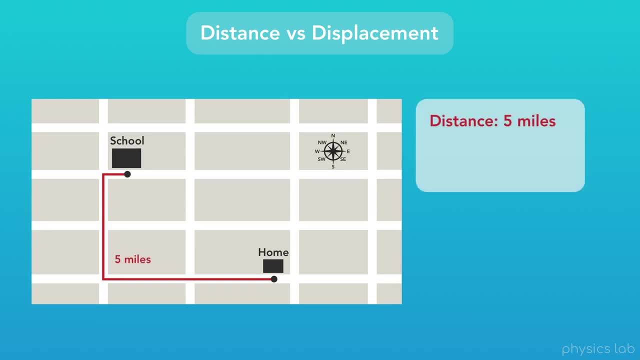 The distance you traveled, let's say, is five miles. What would be your displacement? Well, the displacement is the direct difference between your initial and final points, and we can think of it as an arrow going from your starting point to your ending point. So here, our displacement turns out to be three miles. 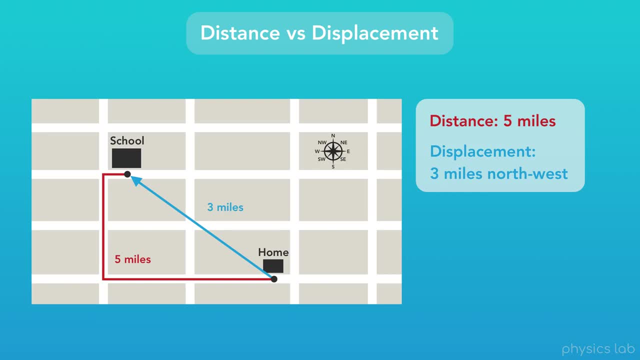 northwest. Displacement is a vector, so it has both a magnitude- three miles- and a direction- northwest. So here's a question for you. Every car has something called an odometer which measures the number of miles driven in your car. If we checked the odometer at home, 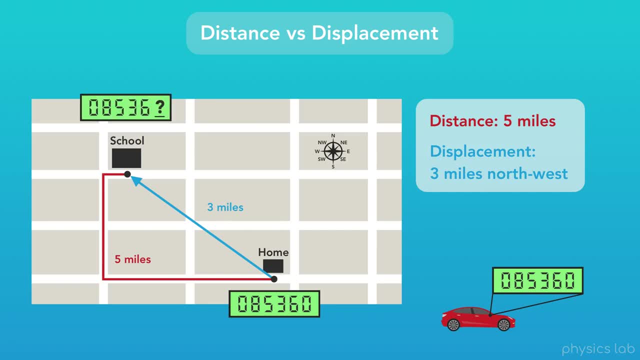 and then checked it again when we got to school. would the odometer increase by five miles or would it increase by three miles? So does the odometer track our distance or our displacement? The answer is yes. The odometer would go up by five miles because it measures distance. It measures the actual path. 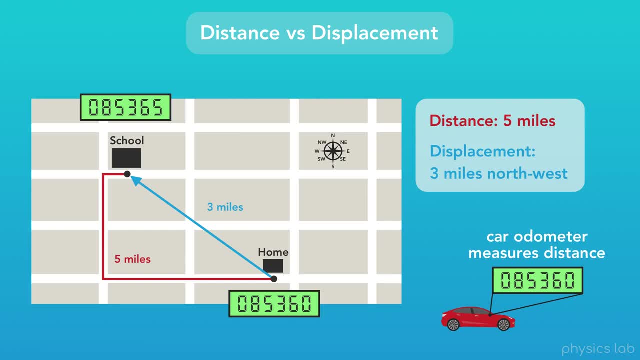 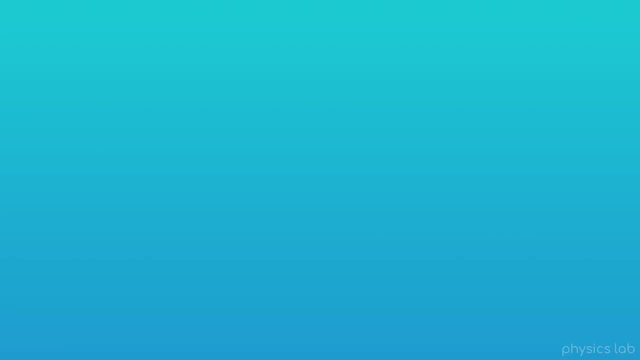 that the car takes. So that's another way to think about the difference between distance and displacement. Next, we can actually use the same examples to compare speed and velocity. Again, Mike walks in a full circle with a circumference of 15 meters. 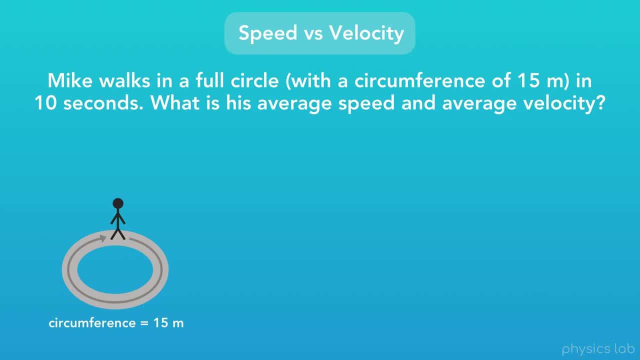 but now we're given that it takes him 10 seconds. What is his average speed And his average velocity? Well, speed is equal to distance over time and his distance traveled is 15 meters and it takes him 10 seconds. So his average speed. 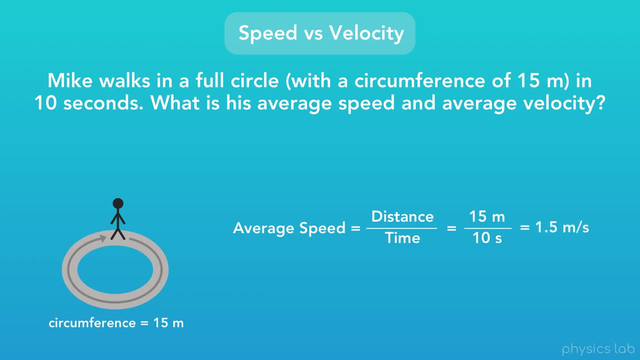 is 15 divided by 10, or 1.5 meters per second. But velocity uses displacement, not distance. We learned last time that his displacement is zero meters, since there's no difference between his initial and final position. So Mike's average velocity is zero meters divided by 10 seconds, or zero meters per second. 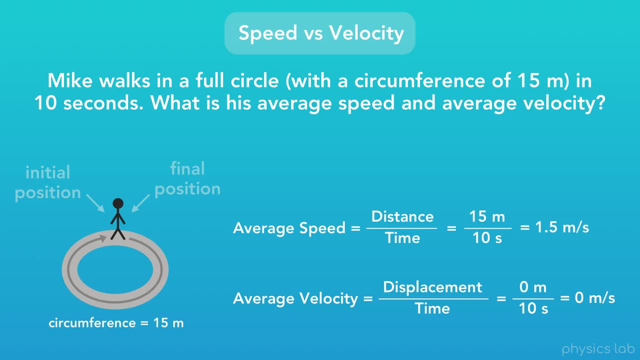 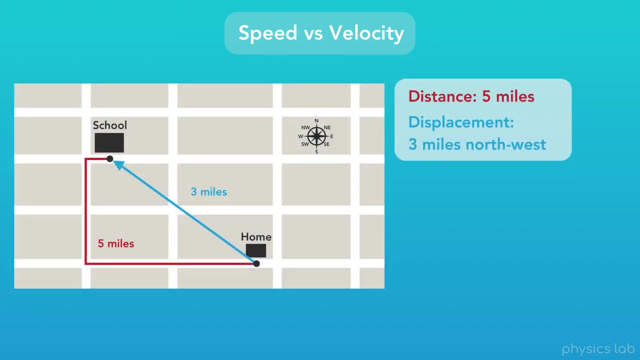 That seems kind of strange because we know Mike was moving as he walked around the circle. But this is how we define average velocity and in this case it's zero. What about our driving example? We already found the distance and displacement of our car. 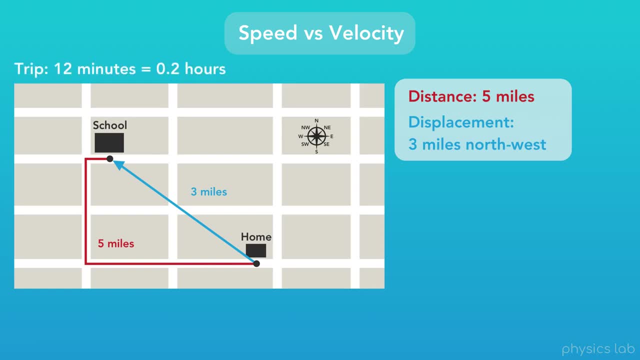 and let's say the trip takes us 12 minutes, which equals 0.2 hours. So what would be our average speed and our average velocity for this trip? Well, speed is distance over time, which would be five miles divided by 0.2 hours. 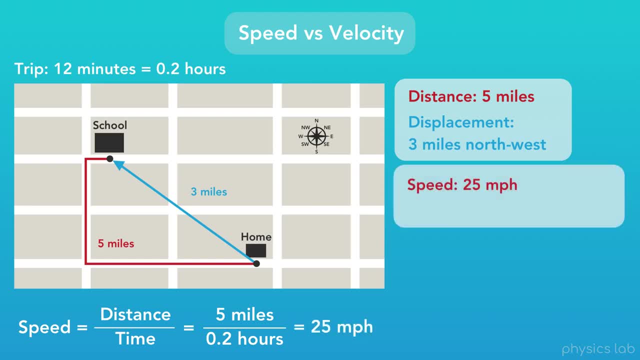 and we get 25 miles per hour. So that's our average speed. Next velocity is displacement over time. So to find the magnitude we would do three miles divided by 0.2 hours, which gives us 15 miles per hour. 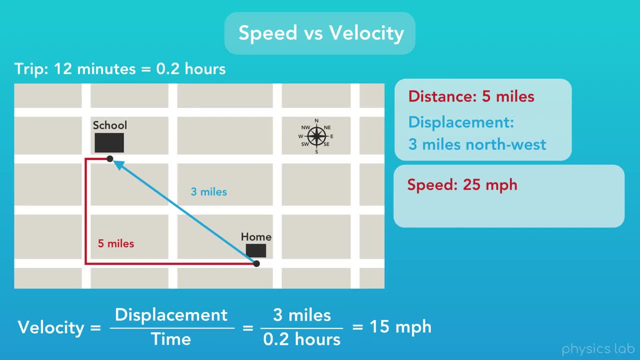 hour. But velocity is a vector so we need to include the direction. So our average velocity would be 15 miles per hour northwest. It has the same direction as our displacement And, similar to last time, every car has what we call a speedometer. That's the thing that tells. 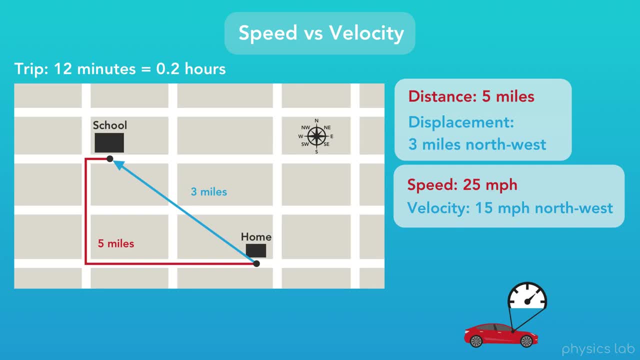 you how fast you're going? Now, does the speedometer tell us the speed or the velocity of the car? Well, the name kind of gives it away, but a speedometer tells us the car's speed. The speedometer only knows we're driving forward, but not which direction we're traveling. 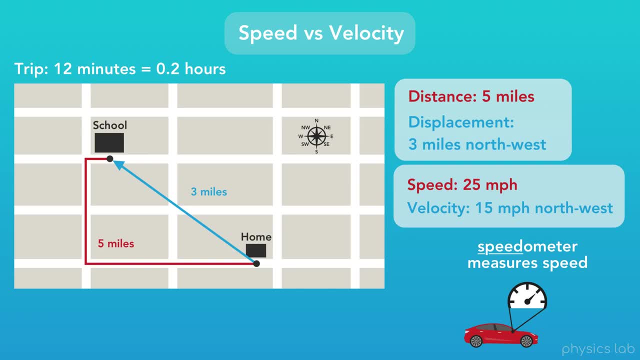 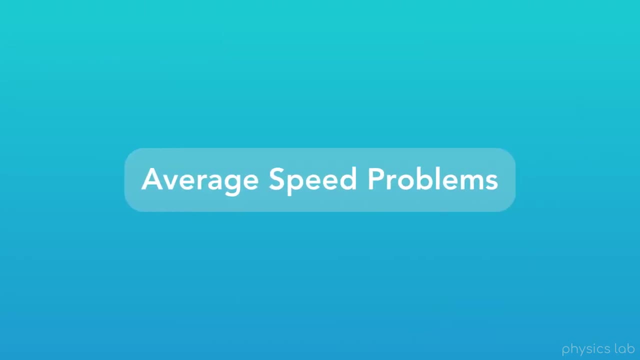 However, if your car has a built-in compass, you could think of combining your speed and your compass direction together to give you your car's velocity, which is a vector. All right, so the last thing we're going to cover in this video is physics problems involving 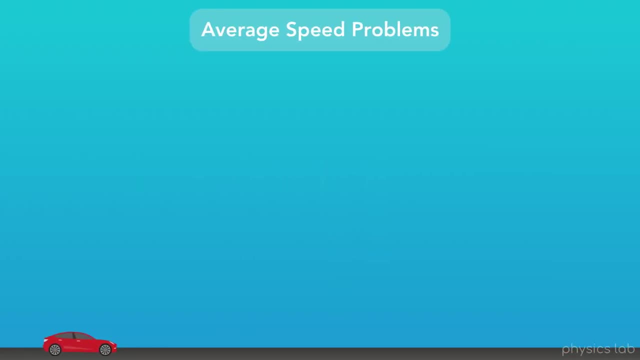 speed. So we're going to talk about speed and then we're going to talk about velocity. So here's our equation for average speed. Average speed equals the total distance traveled divided by the total time it took to travel that distance. I emphasize total because it's an 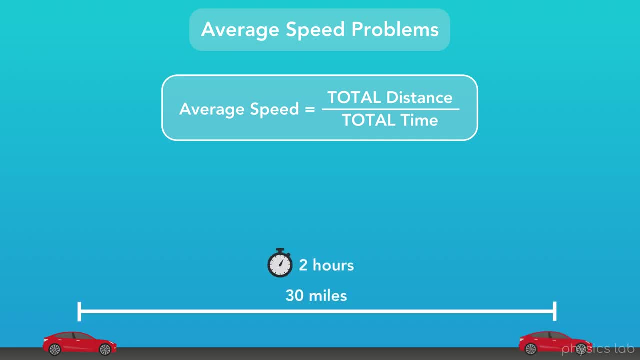 important part of finding average speed. For example, if we said that this car traveled 30 miles and it took 2 hours, then the average speed of the car for that period is 30 miles divided by 2 hours. So if we said that this car traveled 30 miles and it took 2 hours, then the average speed 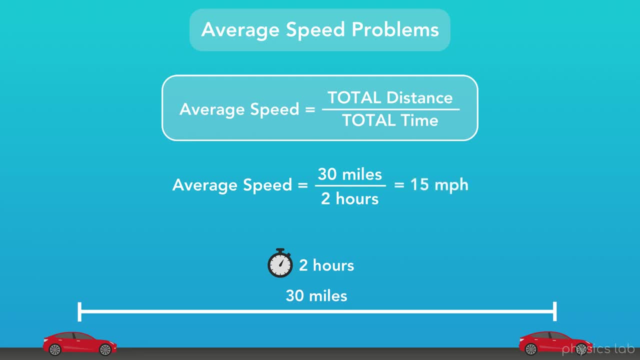 of the car for that period is 30 miles divided by 2 hours or 15 miles per hour. Seems pretty straightforward, right, But sometimes physics problems can trip us up because the information we get isn't this easy And we might forget that average speed is defined. 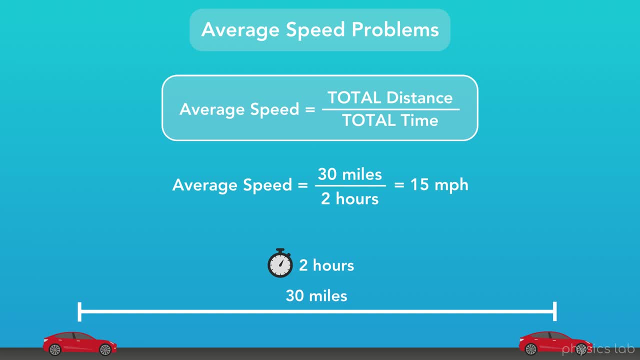 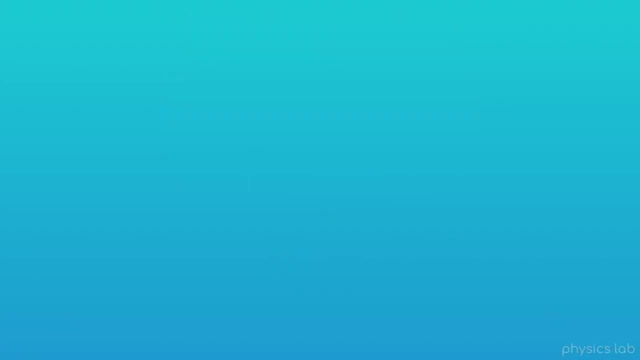 as the total distance over the total time. If the problem wants us to find average speed, this is how we have to calculate it. Take a look at this example: A car drives 150 miles at 50 miles per hour, then drives for another 150 miles at 75 miles per hour. What is the average speed of the? 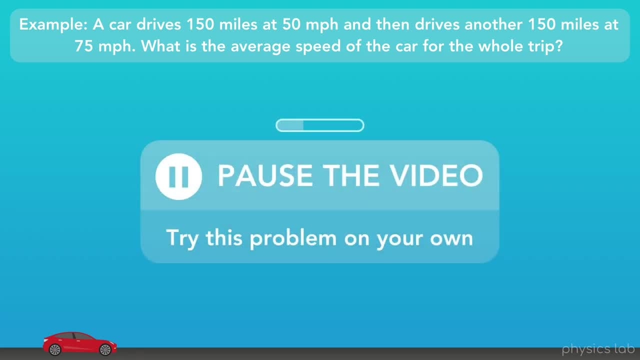 car for the whole trip. So what are the important pieces of information in this word problem? We're given some numbers: The car drives 150 miles at 50 miles per hour and 150 miles at 75 miles per hour And we're being asked to find the average speed. So we see the word average. 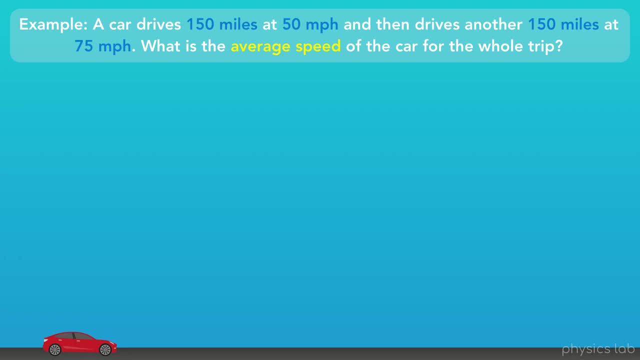 We know what average means. We know how to take a group of numbers and find the average right. So to find average speed, can we just find the average of 50 miles per hour and 75 miles per hour? That would be 50 miles per hour plus 75 miles per hour divided by 2,, which gives us 62.5. 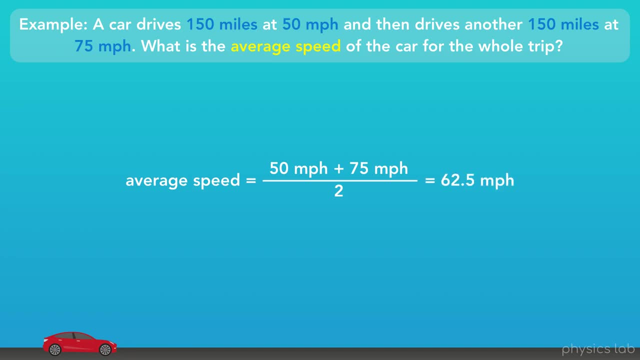 miles per hour And we're being asked to find the average speed of the car for that period, So we can find the average speed of the car. That seems logical, right? Well, this is actually not the average speed. Remember, this is how we define it. The average speed equals the total distance. 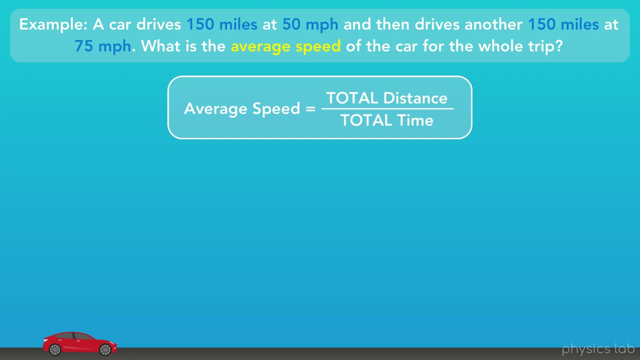 divided by the total time. So we know the total distance. 150 miles plus 150 miles gives us 300 miles, But we don't know the total time. How can we find it? Well, we know the distance and the speed of the car for each part of this trip, So what we can do is find. 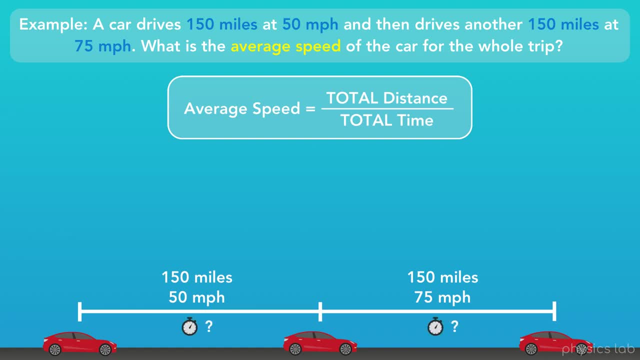 the amount of time the car traveled for each part of the trip and then add them together to get the total time. So speed equals distance divided by time. But we want to rearrange this equation so we can find time. If we multiply both sides by time, we get speed times. time equals distance. 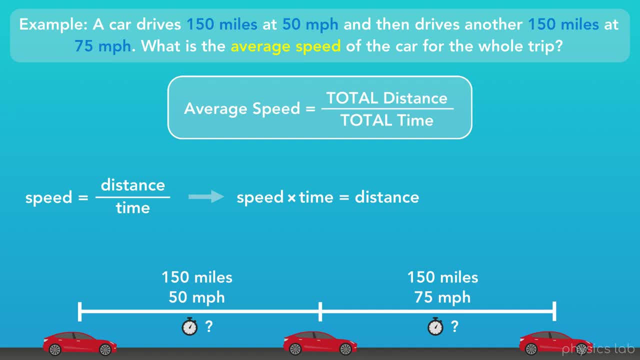 If we divide both sides by speed, we get time equals distance divided by speed. Quick side note: we just rearranged our equation, so time is by itself on one side And then next we're going to plug in numbers to solve for time. 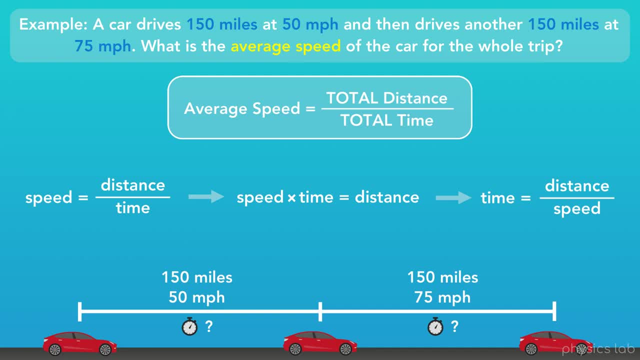 We could have also plugged in numbers first and then rearrange the equation for time. I just chose to do it this way. Okay, so for the first part of our trip, we have 150 miles divided by 50 miles per hour, which equals 3 hours. For the second part of the trip, 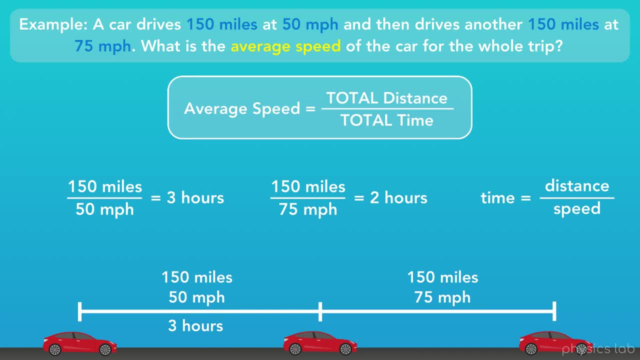 we have 150 miles divided by 75 miles per hour, which equals 2 hours. So the total time for the entire trip is 3 plus 2, or 5 hours. Now we can calculate the average speed of the car for the entire trip. Average speed equals the total distance: 300 miles divided by the total time. 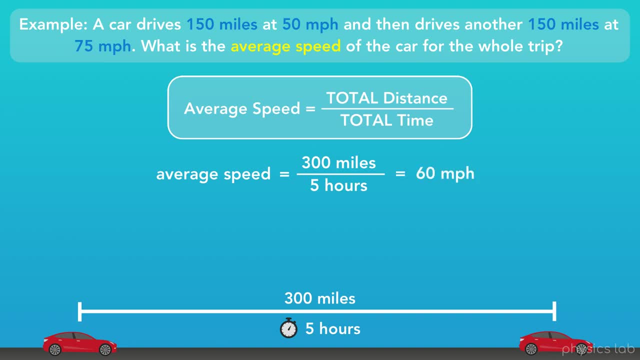 or 5 hours, which equals 60 miles per hour. So that is the actual average speed that this problem is asking us to find. So why is this answer correct and why is it different than the one we got before? Let's explore this for a minute. You don't need to remember this, but I think it'd. 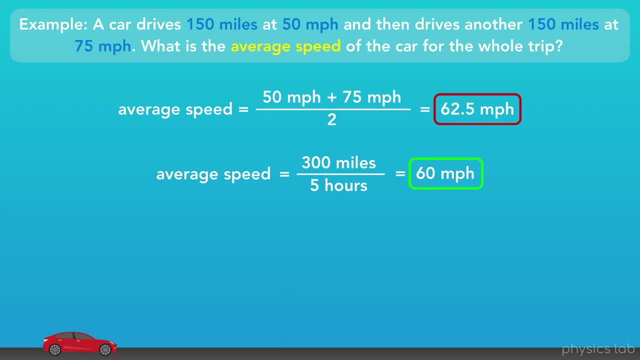 be nice to clear things up. So this first method of finding average speed feels right, doesn't it? 62.5 is halfway between 50 and 75,, which is how we're used to finding the average of two numbers, But the correct average speed, 60,, is less than that. It's closer to 50 than it is to 75.. 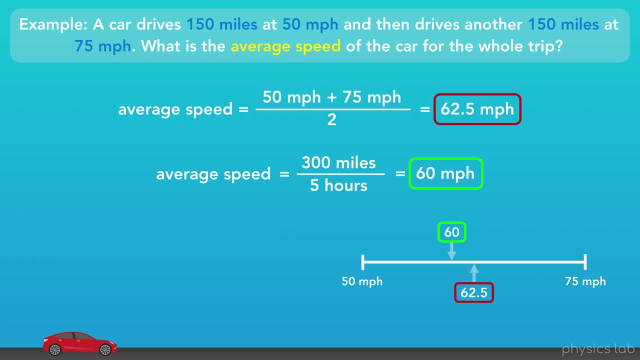 So why is that? The car even drove the exact same distance at each of these two speeds. So it feels like each speed is equally important. Like if you imagined a balance, each speed would have equal weight. Now if, instead, the car had driven 50 miles per hour for 1000 miles? 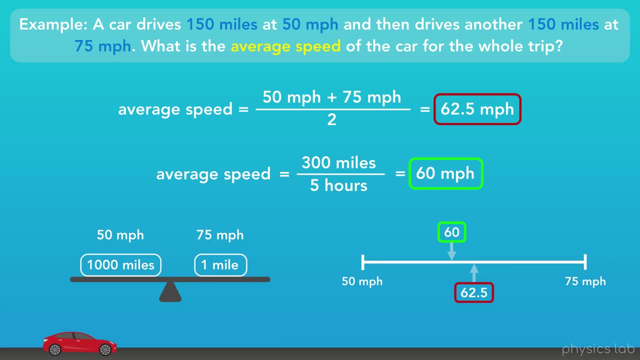 and 75 miles per hour for only 1 mile. then it would feel like the 50 miles per hour would hold more weight and the average should be closer to 50. But the distances are actually the same. However, the times are not the same. We found that the car was driving 50 miles per hour for 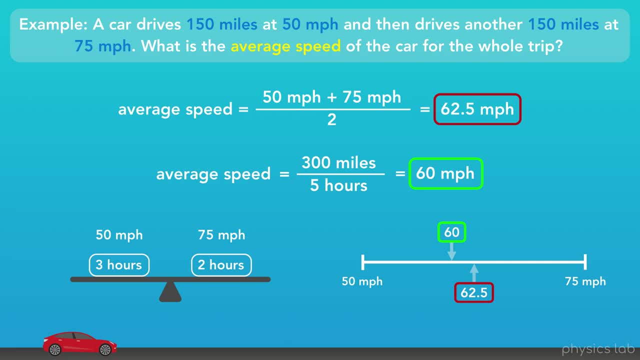 3 hours and 75 miles per hour for only 2 hours. So since the car was driving at 50 miles per hour for a longer time, the 50 has more weight to it, so the average speed is closer to 50 than 75.. 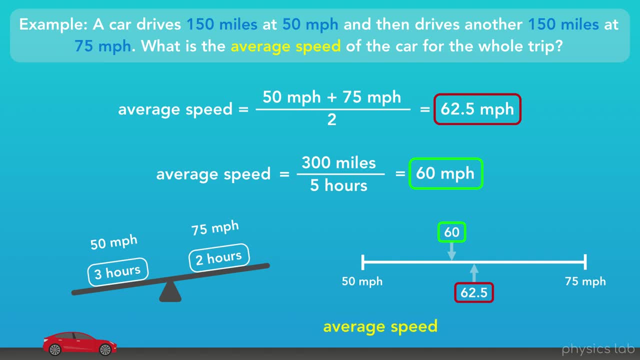 So, really, when we say average speed, in physics you could think of it as the time-weighted average speed, as opposed to the distance-weighted average speed. When an object, like a car, travels at different speeds over its journey, we're averaging the speeds based on their times and not on their distances. 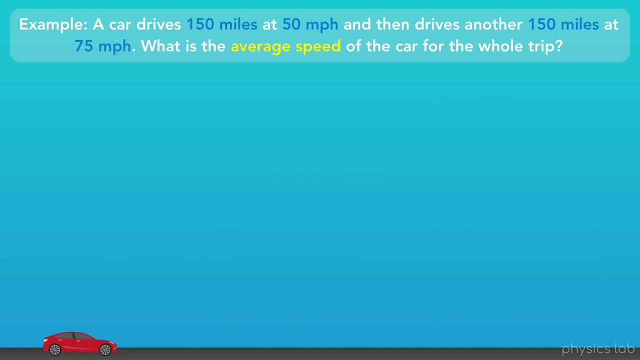 Anyway, you can forget about that. The nice thing is, all you need is this equation: If a problem asks you to find the average speed, just divide the total distance by the total time and you'll be good to go. Alright, let's do a recap of what we learned in this video. 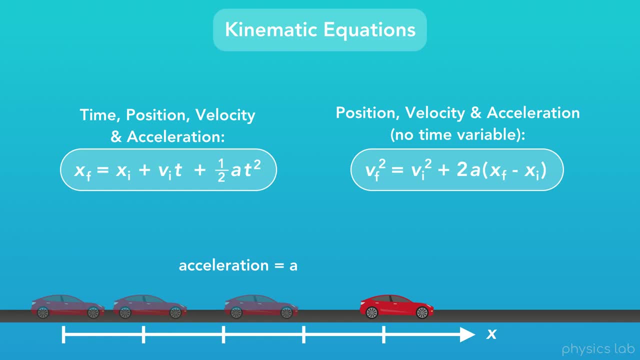 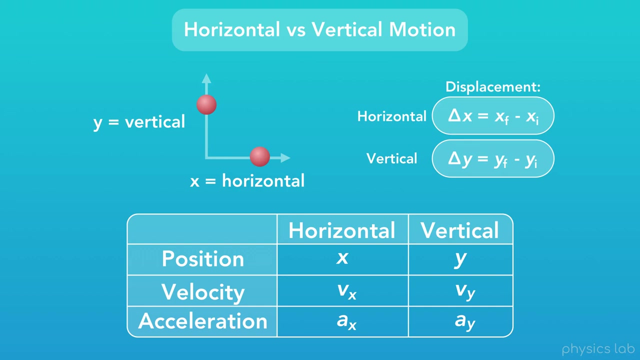 First off, we learned the last two kinematic equations for a linear motion, which both apply to an object that's accelerating. Next, we learned that we can describe horizontal motion using the variable or the subscript x, And we describe vertical motion.